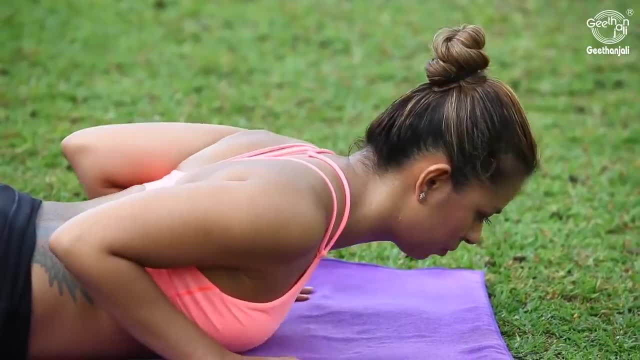 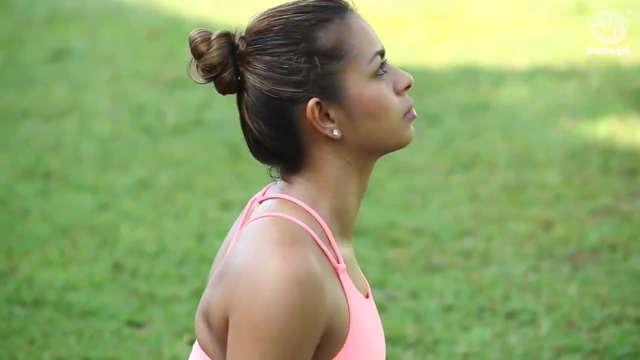 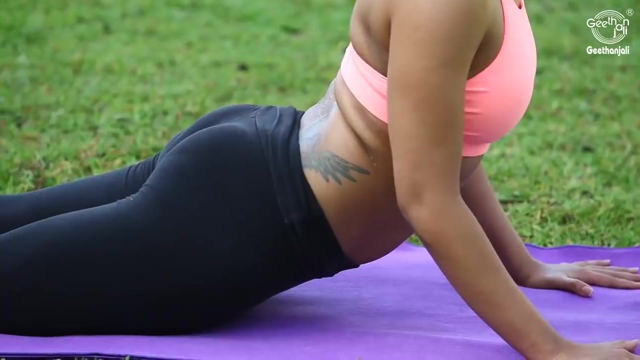 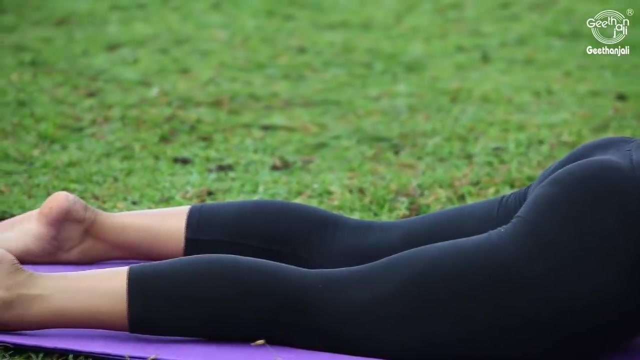 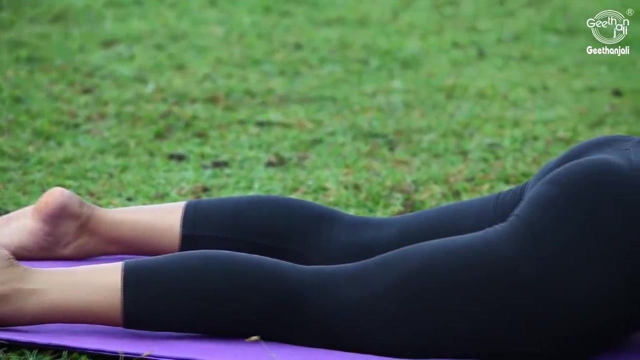 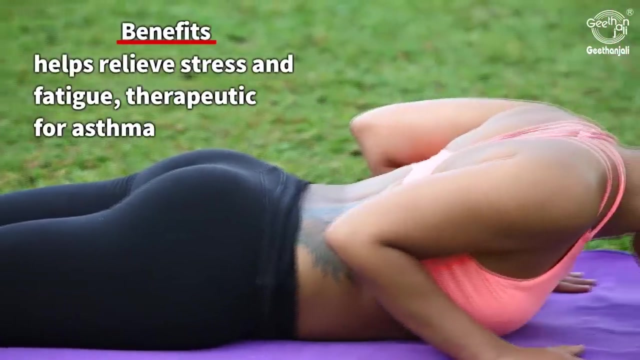 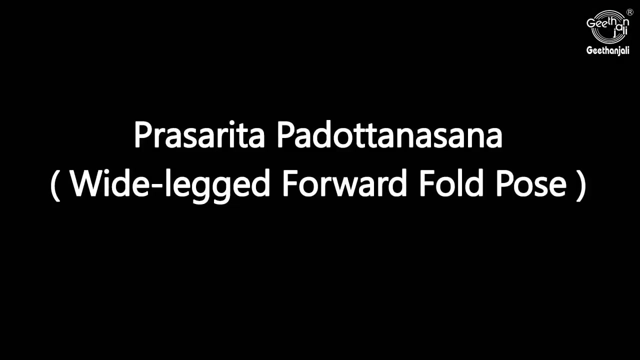 Gently raise the body up, resting the palm on the floor like a cobra rising up. Stay in that position for a while and resume previous position with face down. Benefits: Helps relieve stress and fatigue. Therapeutic for asthma. stand up with legs wide apart on the sides placing the hand on your 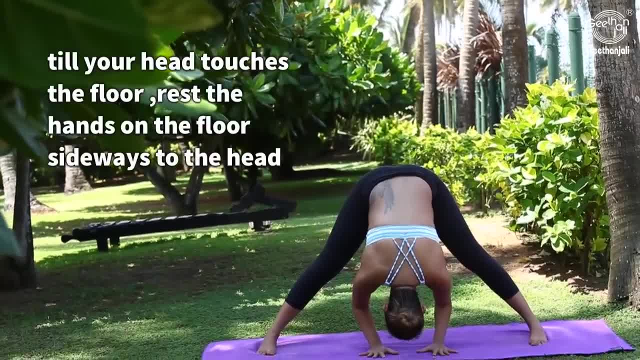 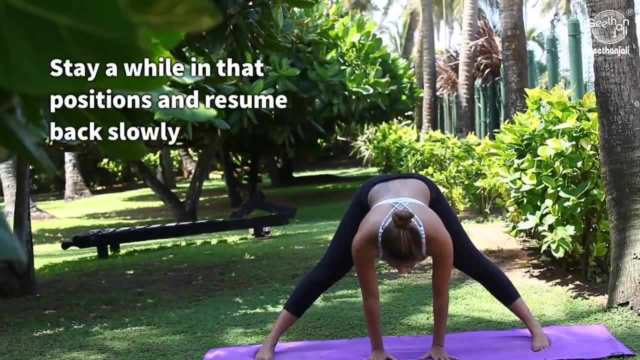 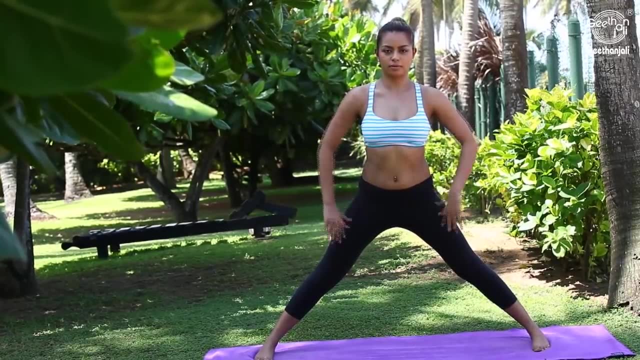 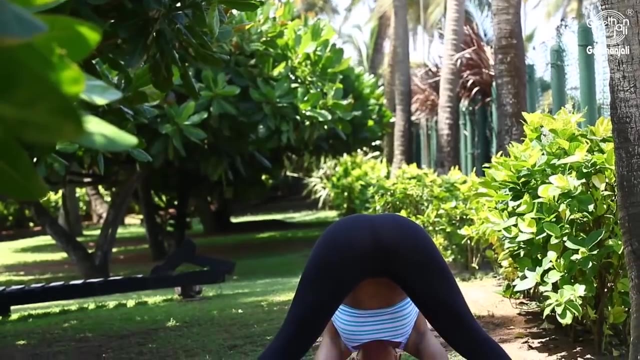 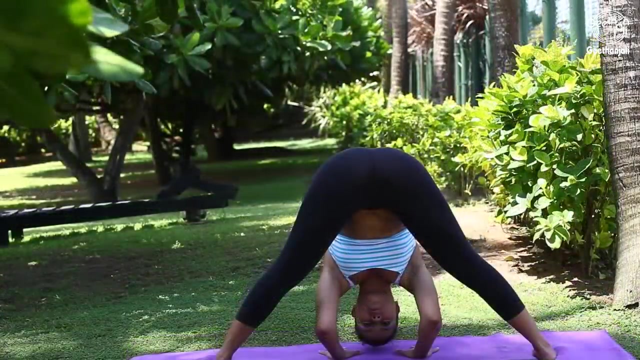 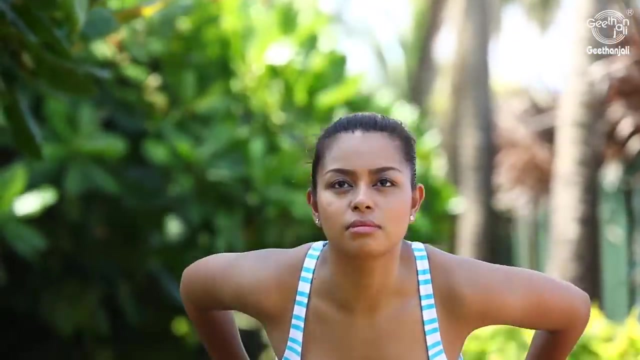 hips slowly bend forward till your head touches the floor. rest the hands on the floor sideways to the head. stay a while in that position and resume back slowly. repeat this three times. stand up with legs wide apart on the sides, placing the hand on your hips. slowly bend forward till your head touches the floor. rest the hands on the. 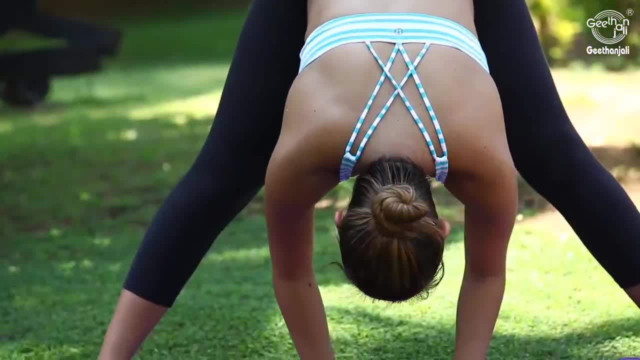 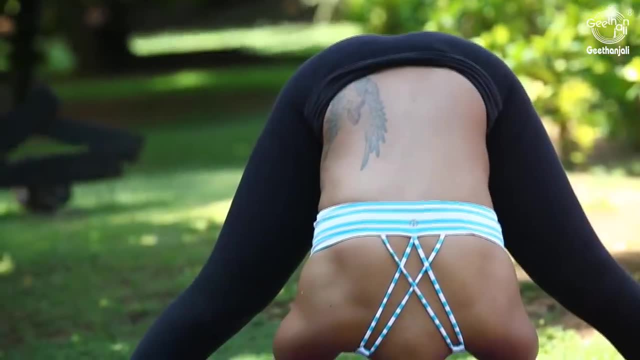 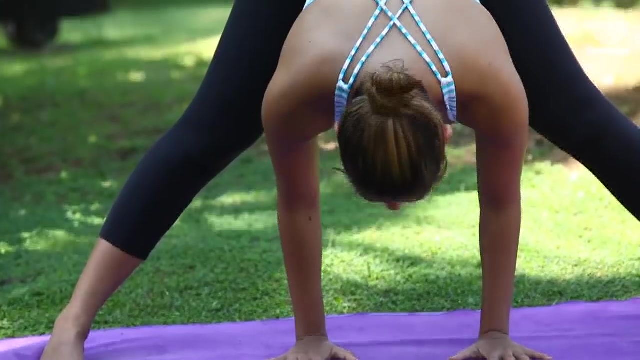 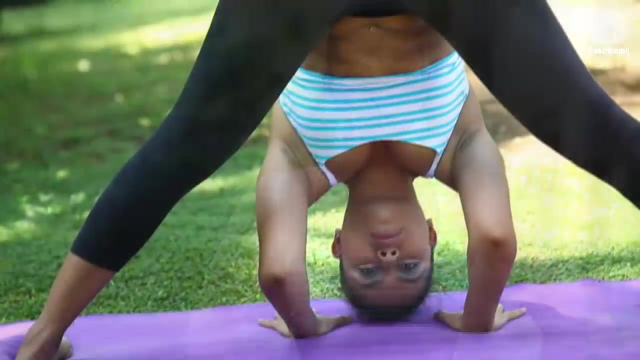 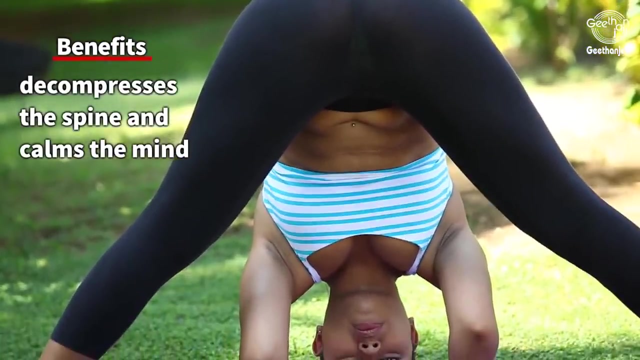 floor sideways to the head. stay a while in that position and resume back slowly. repeat this three times. benefits stretches groins, hips and hamstrings. decompresses the spine and calms the mind. benefits stretches groins, hips and hamstrings. decompresses the spine and. 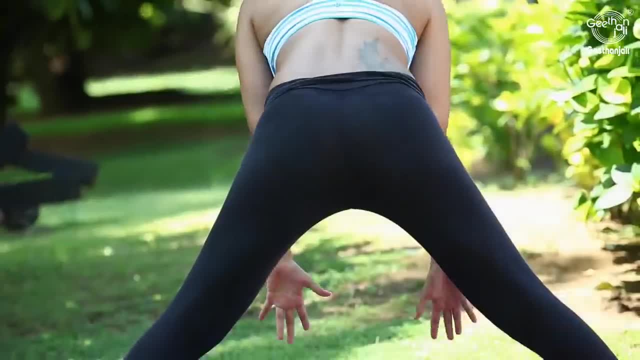 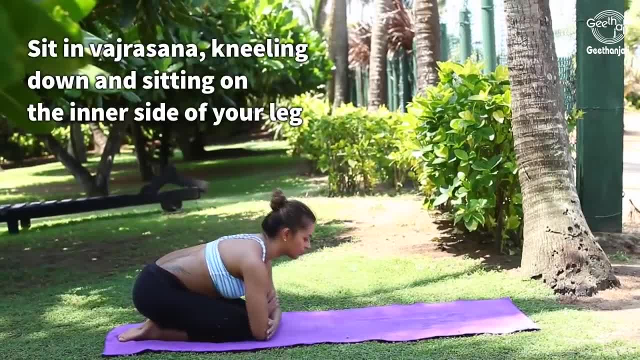 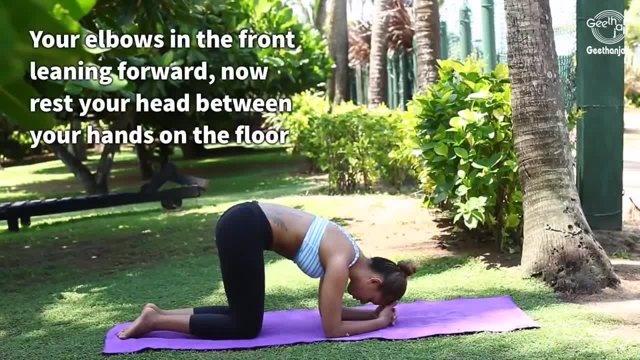 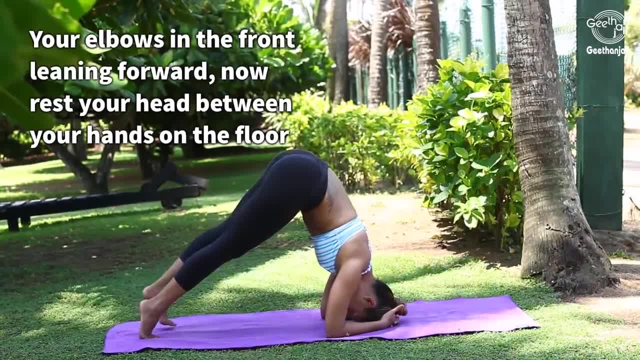 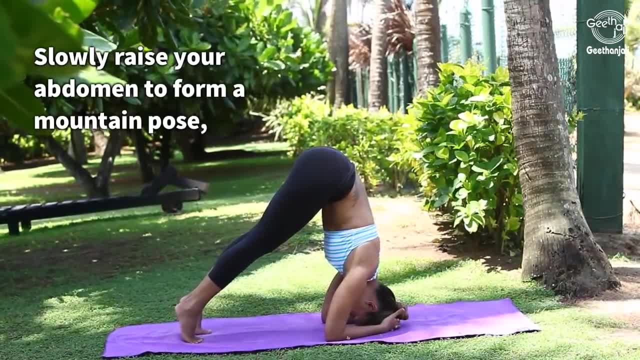 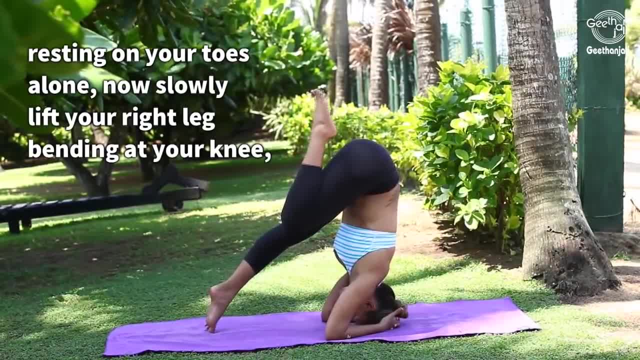 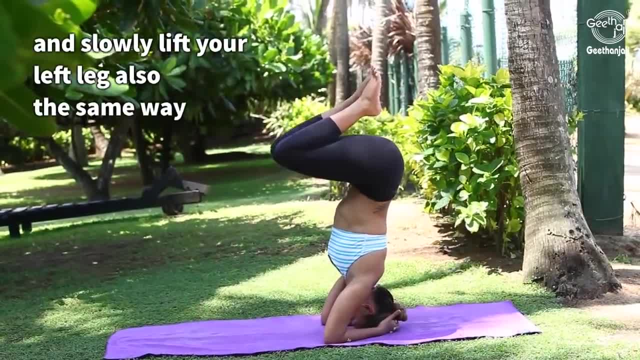 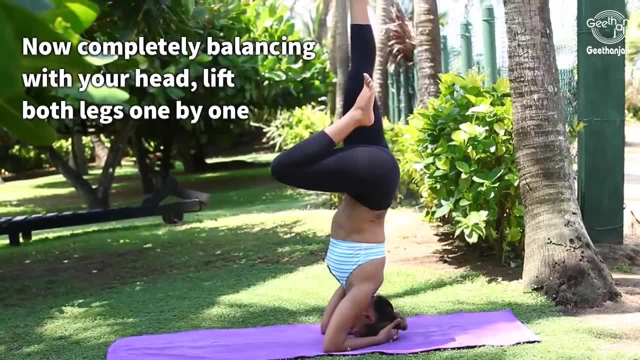 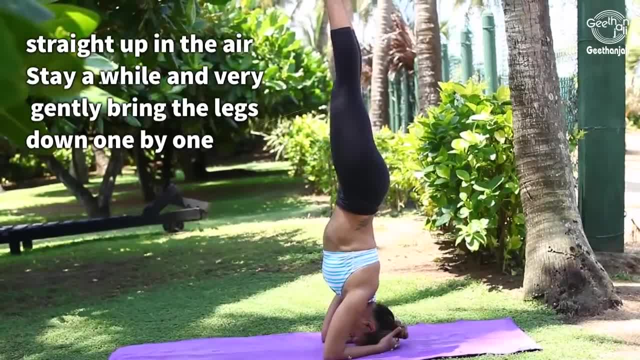 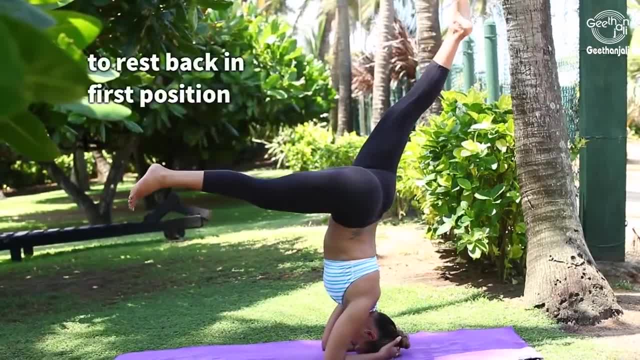 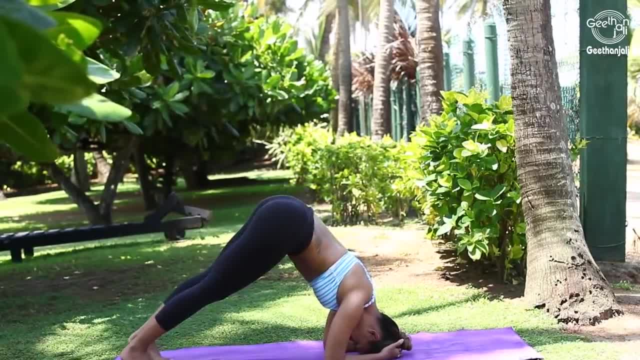 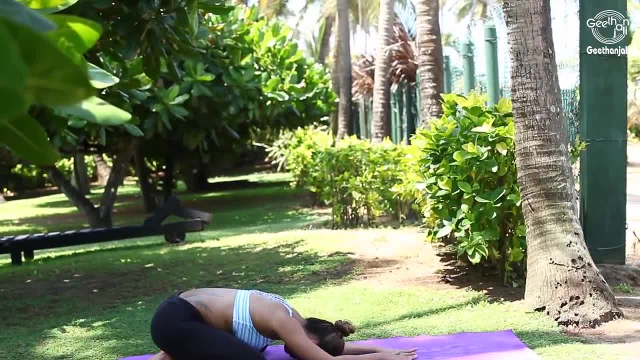 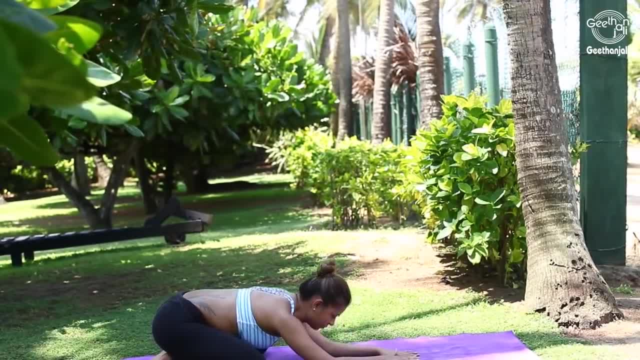 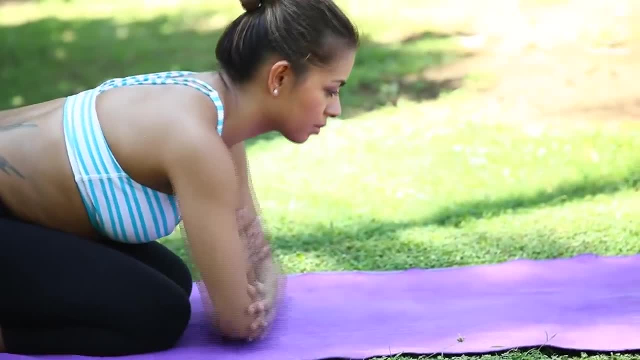 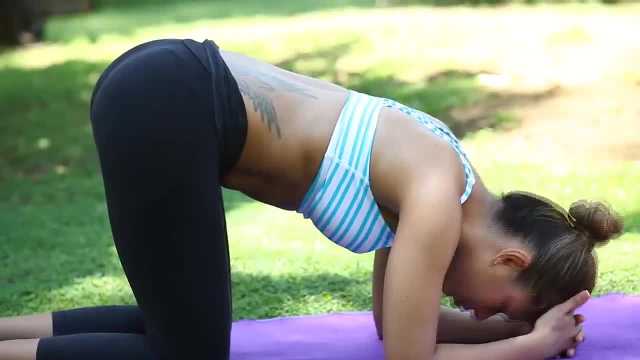 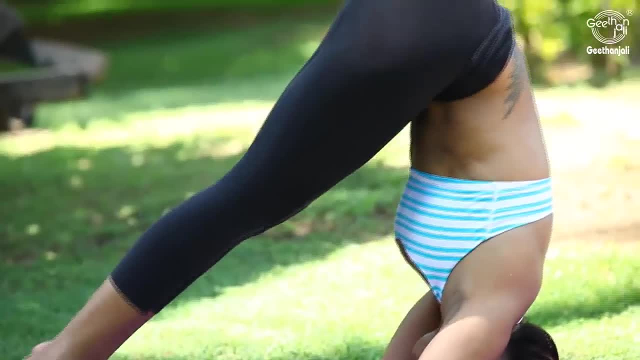 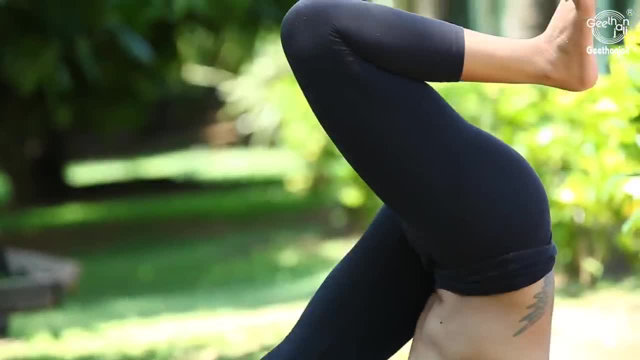 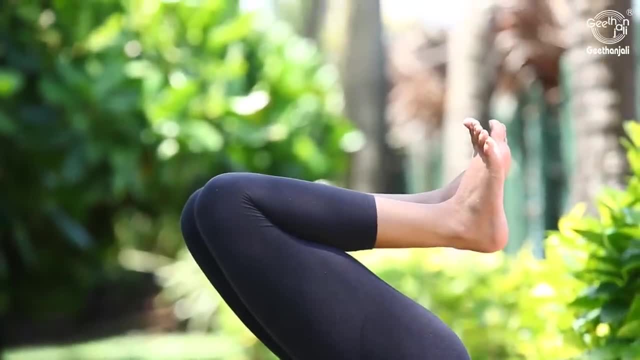 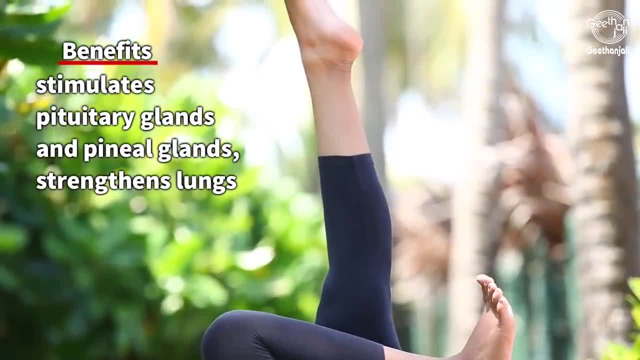